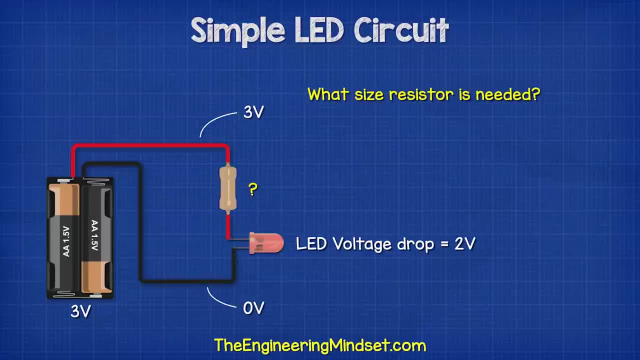 a voltage drop of around 2V, and so our resistor needs to remove the remaining voltage. So 3V subtract 2V equals 1V. We know the LED needs a current of around 20mA. So 1V divided by 0.02A. 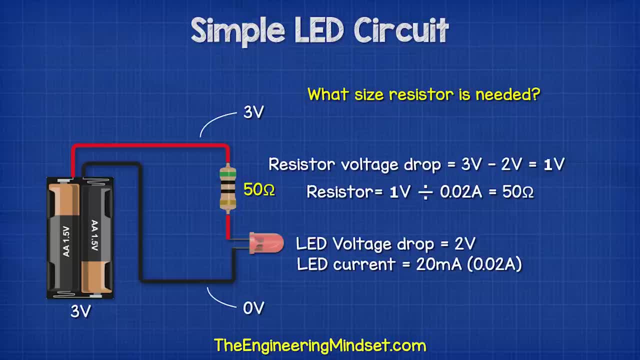 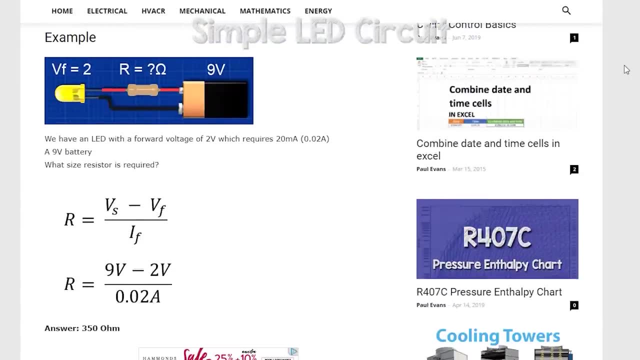 equals 50Ω of resistance. Make sure you convert your mA to amps for this calculation To make it easier. we do have a calculator on our website where you can just input your values. I'll leave a link in the video description down below for that. 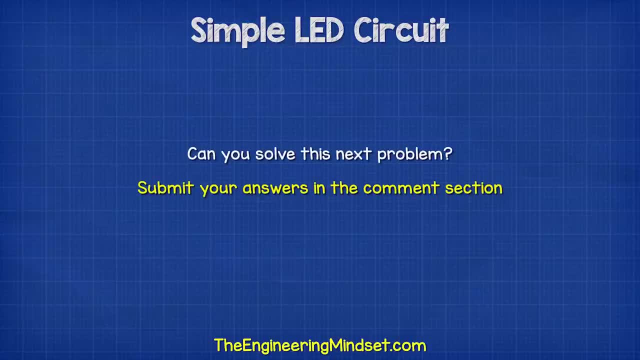 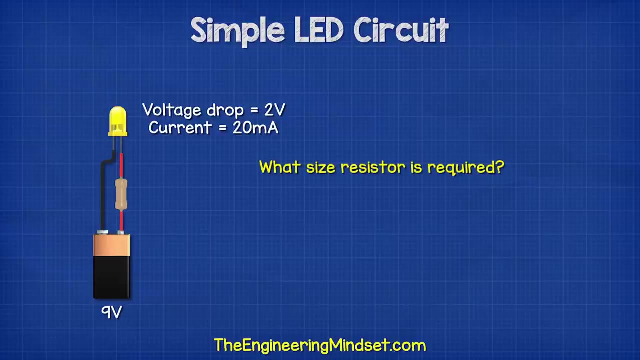 Ok, now you try to solve this one. before I do, Let me know your answers in the comment section down below. Let's say we have a 9V battery and we want to connect a yellow LED which has a voltage drop of 2V and requires 20mA of current. So what size resistor is required? 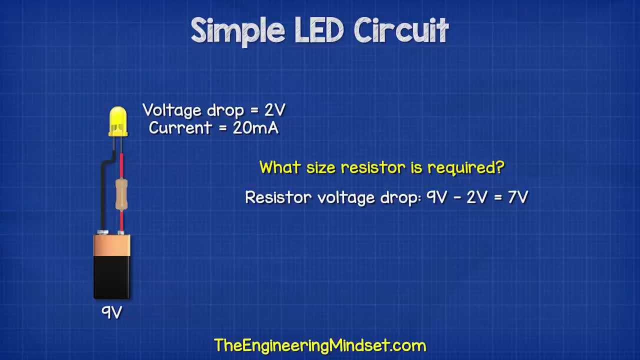 Well, we have a 9V supply, so subtract 2V for the LED and that leaves us with a 7V drop for the resistor. The current is 20mA, so 7 divided by 0.02A equals 50Ω. 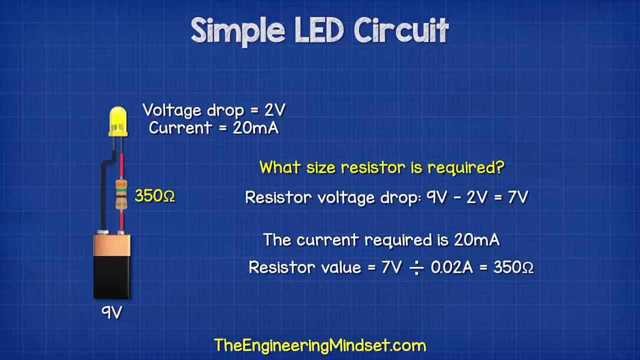 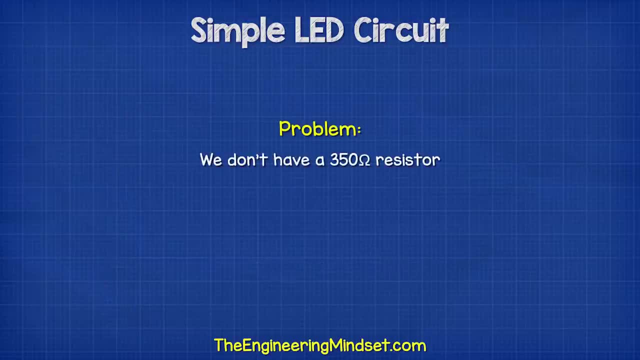 Now the problem is that we don't have a 350Ω resistor. We only have a 330Ω or a 390Ω, So which one should we use? As we saw earlier, we need to ensure the current doesn't exceed 20mA. 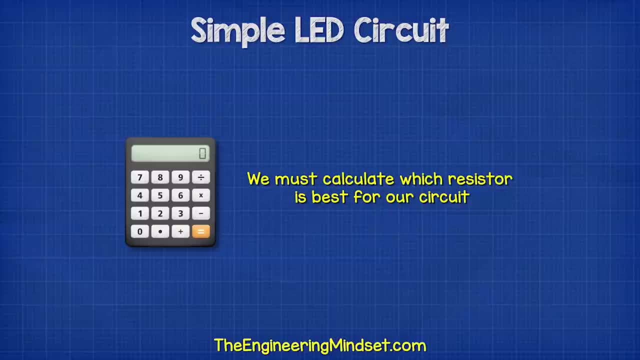 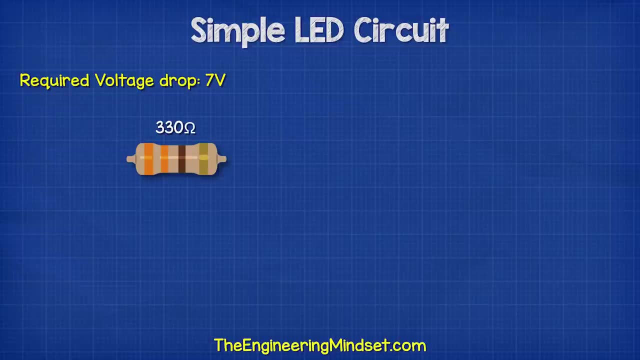 So we will have to calculate which resistor suits us best. To do that, we just divide the required voltage drop of 7V by the resistor value of 330Ω to get 0.021A. And then, if we do the same, 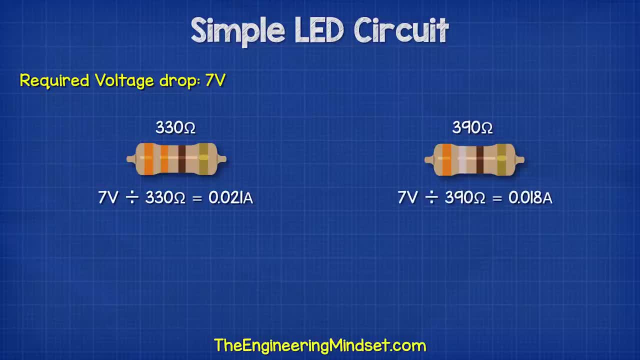 for the 390Ω resistor, we will get 0.018A. Both of these values are very close and they both will work, But to be safe, we will choose a 390Ω resistor, as our LED will therefore last longer.